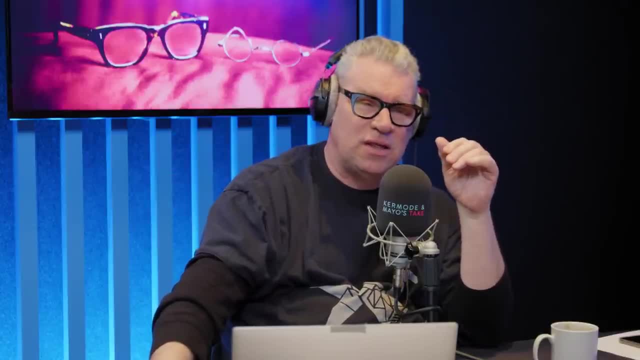 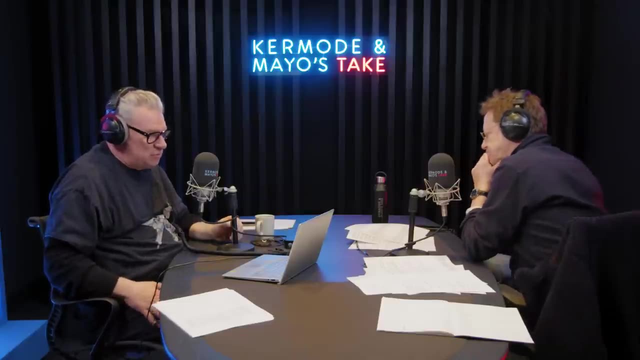 Toby says: can you just give yourself the night off? And he goes. you wouldn't say that to an Olympic athlete. I mean you might. And then, brilliantly, as I've said, I mean you can see the film yourself and enjoy it. 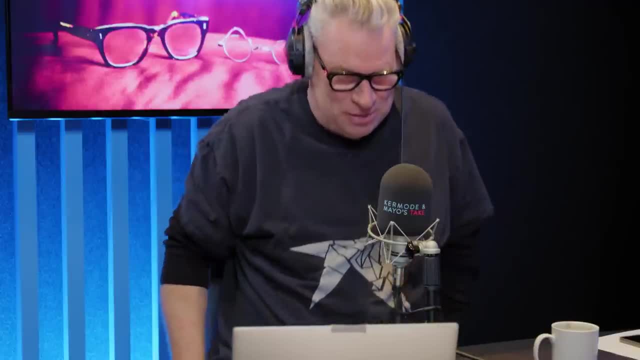 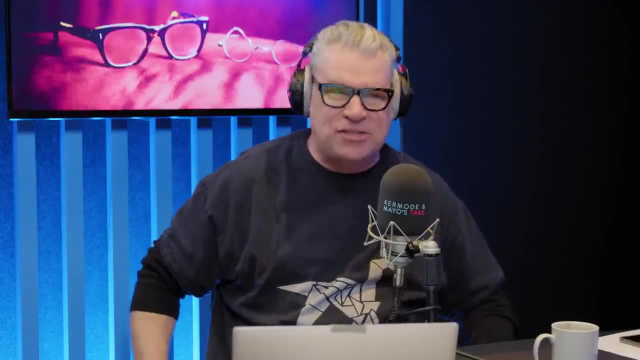 but there's a brilliant bit where Toby turns up to something and Robert Fripp says: you have just missed a meeting which was the most important meeting in the entire history of the band. so this film is completely worthless. And then walks out Fantastic. 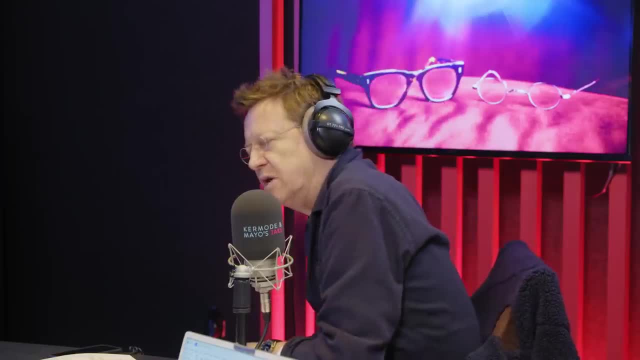 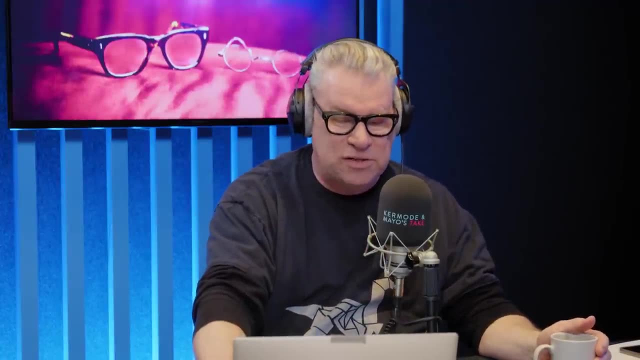 It's great, It's really really good fun. And do you like? Is it worth watching if you don't care at all about It? is? And the answer to that is: I watched it with a good lady professor her indoors who could not care less about King Crimson. 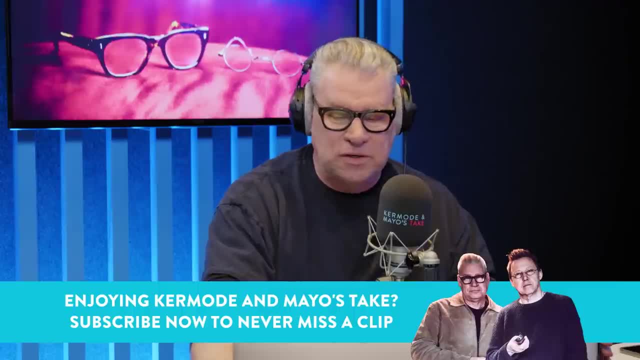 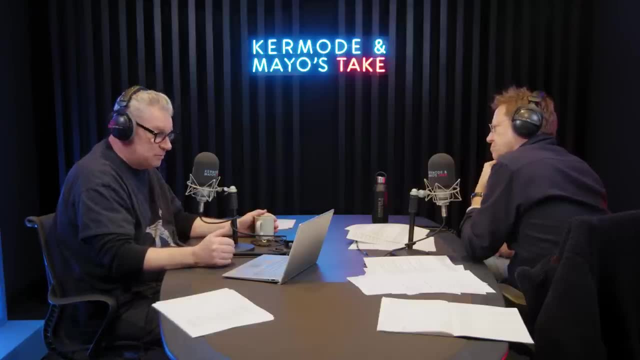 I like King Crimson. King Crimson- up to a point I think you know Lark Tongue's an aspect and all that, but the very first time I was ever on camera, because I grew up in an age in which people didn't have video cameras- 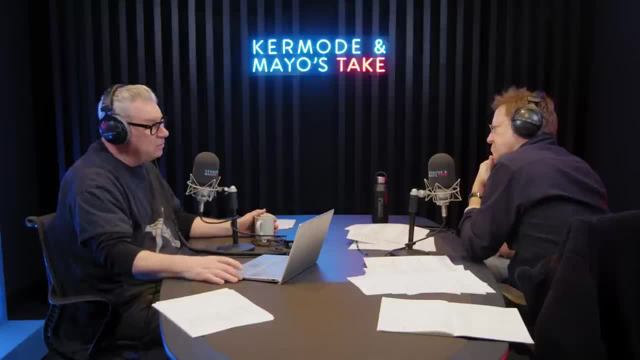 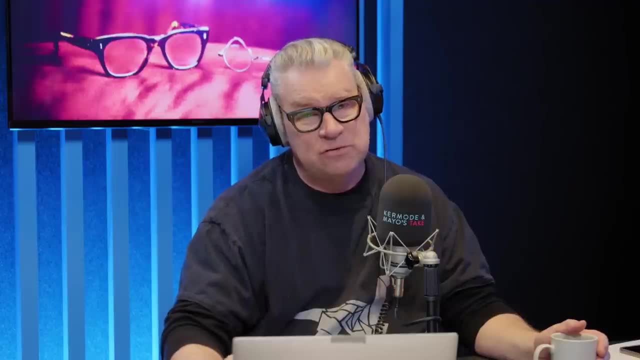 as did you, And when I was at Manchester University, there was a guy who was a drama student whose project it was to make a music video, And he made a music video for Talon Jinji in which he had this little sort of drama thing. 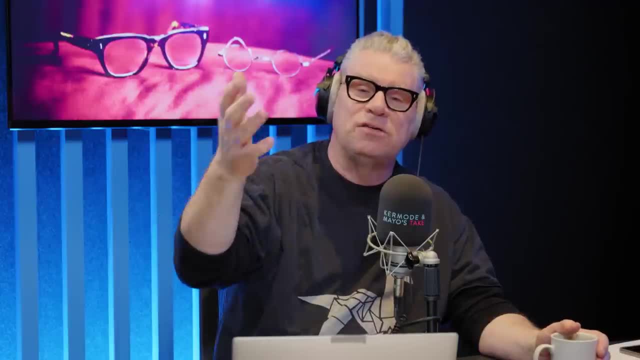 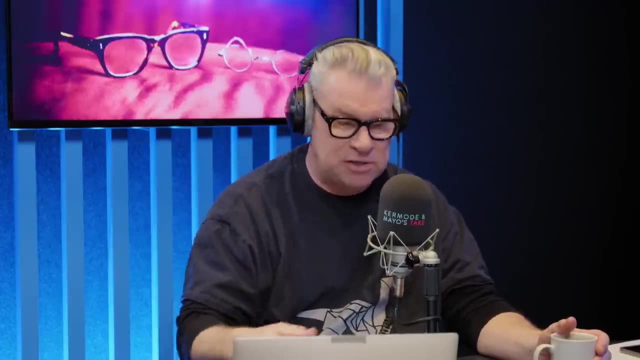 And I had to lip sync the interview in which the guy talks about this is a dangerous place. this is a dangerous place, And it turned out. that was when I discovered I could lip sync- Not lip sync, singing it's lip sync dialogue. 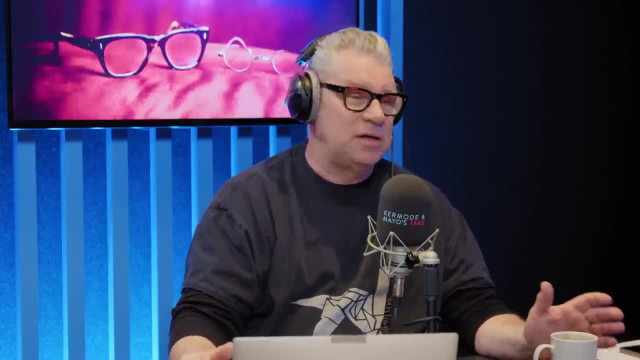 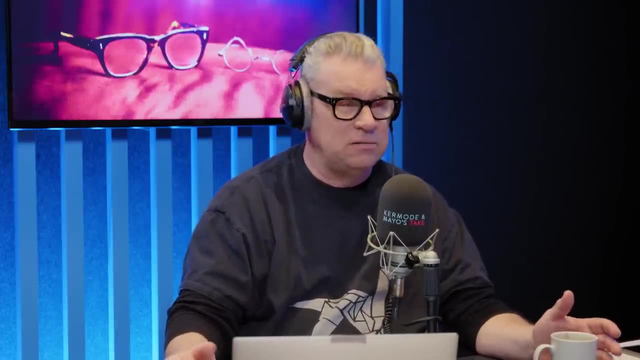 And here's a weird thing: I'm not very talented in many ways at all, but it turns out I can lip sync dialogue really well. I'm very good at ADR and I can ADR Rerecording, like when you and I recorded a thing. 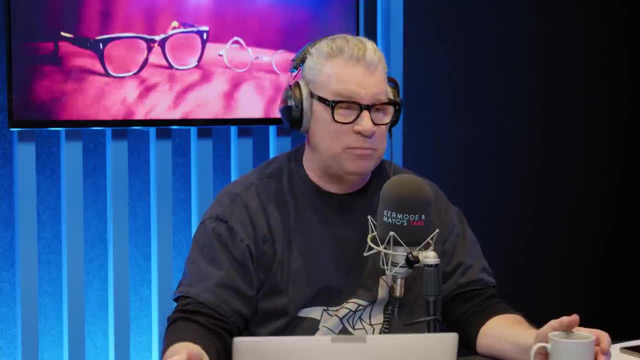 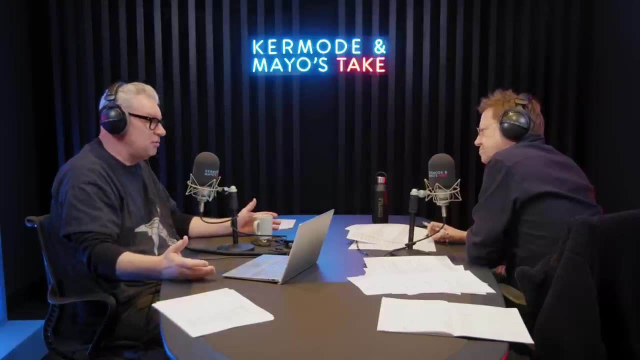 Remember, we turned up at a train station to record an advert for a show and there was like 400 people, but somehow the sound didn't work And then we had to dub ourselves back in again. Well, it turns out. It turns out, this is a completely useless skill. 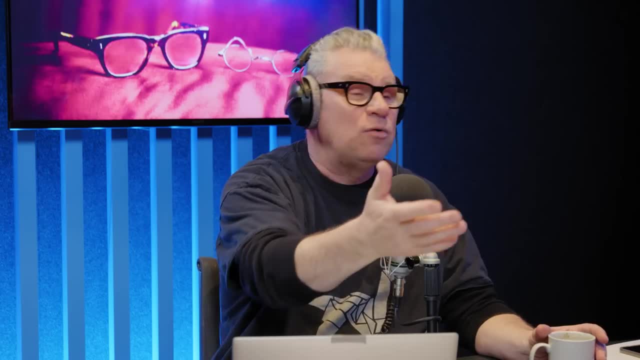 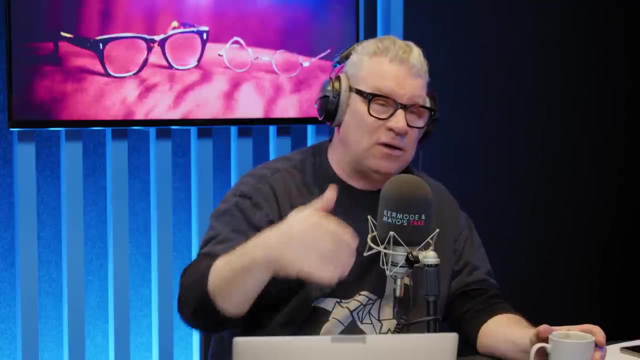 outside of a very specific area. You've got it. You know what Mark Jenkin does when he makes his films. He doesn't record the sound and then all the actors dub themselves back in again afterwards. Mark actually deflated me. He said it's not a skill. most people can do it.